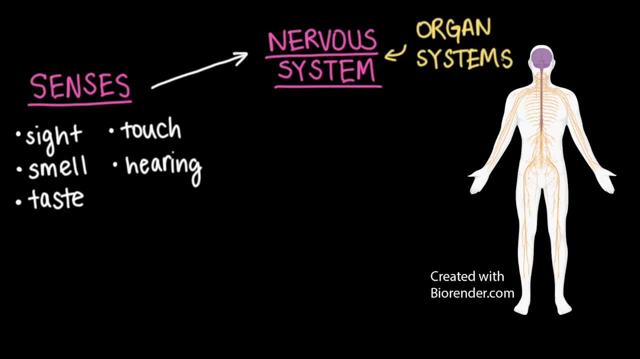 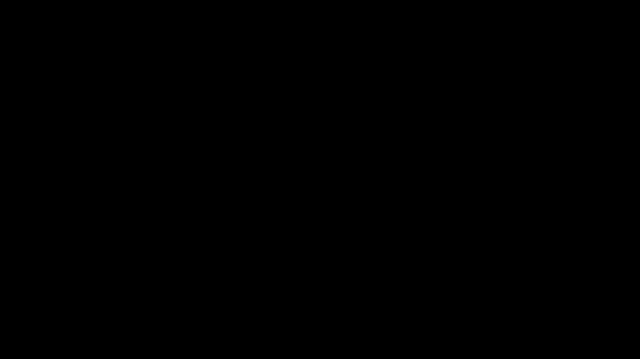 complex organ systems that work together to perform all different kinds of functions. Today, let's talk specifically about the nervous system, which is an organ system that allows us to sense and respond to our environment. To begin, the nervous system contains specialized cells and. 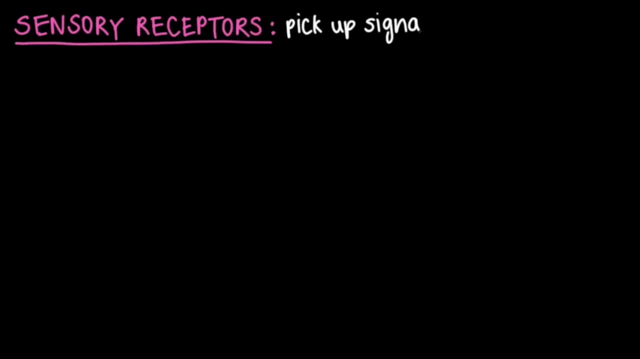 cell parts, called sensory receptors, which are able to pick up signals from the environment. These signals are called stimuli, or stimulus, if you're talking about just one. Stimuli can come in many different forms, For instance, mechanical stimuli are physical in nature and are involved with our senses of touch and hearing. You can strum a guitar. 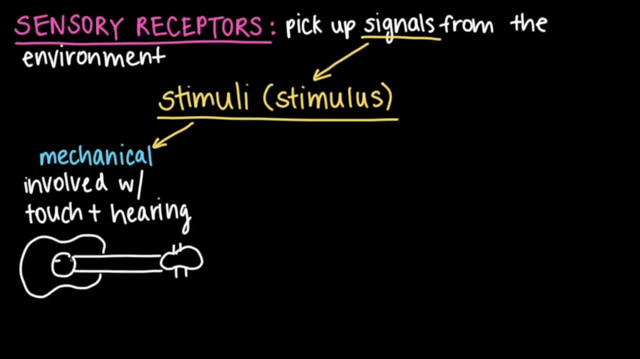 feeling the strings against your fingertips and listening to the unique tones it produces as the strings vibrate. Those are all mechanical stimuli. Chemical stimuli are made up of molecules and are used to make sounds. They are also used to make sounds. They are used to make sounds. 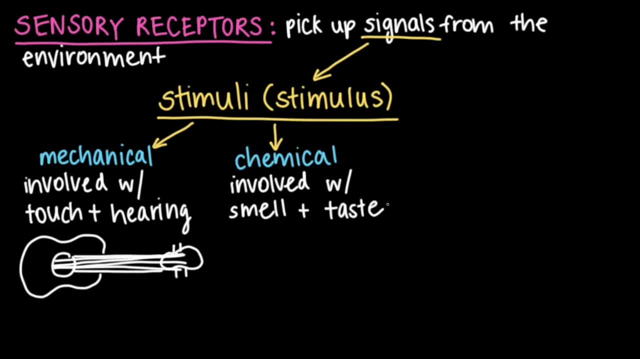 are involved with our senses of smell and taste. To illustrate an example, imagine eating a tasty bowl of chicken noodle soup. As you spoon mouthfuls of soup into your mouth, your taste and olfactory receptors are flooded with molecules that signal the qualities of the food you're eating. These 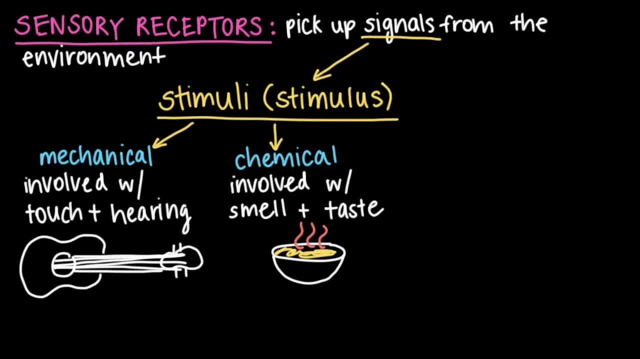 molecular signals are chemical stimuli and in this case, the molecules from the chicken noodle soup convey that the food you're eating is savory and extremely delicious. Basically, electromagnetic stimuli are involved with our sense of sight and include the light that comes into our eyes every day, the sunlight that makes you squint, the traffic lights you see. 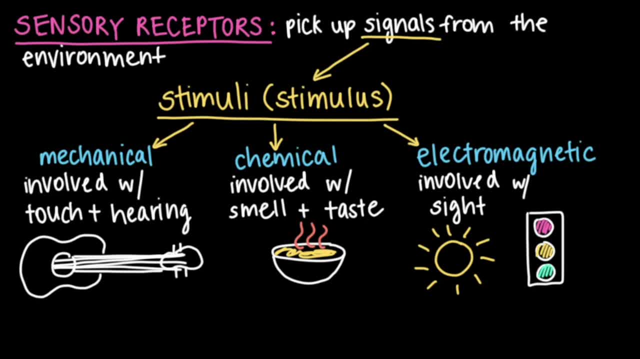 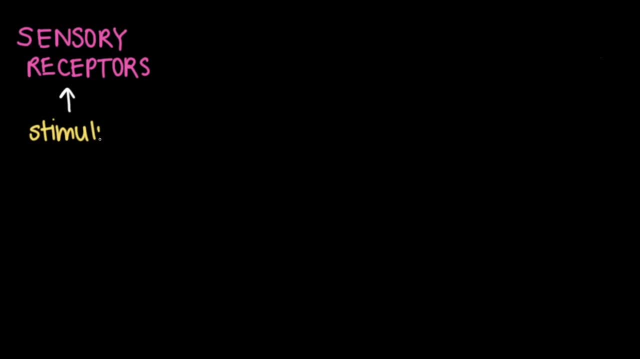 on the street and the vibrant and diverse colors all around you. These are just a few examples of electromagnetic stimuli in the form of light. So then, what happens after sensory receptors detect stimuli? Well, once a sensory receptor receives the information, it passes this information along. 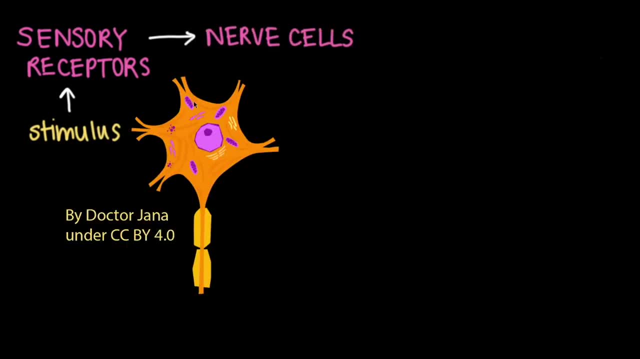 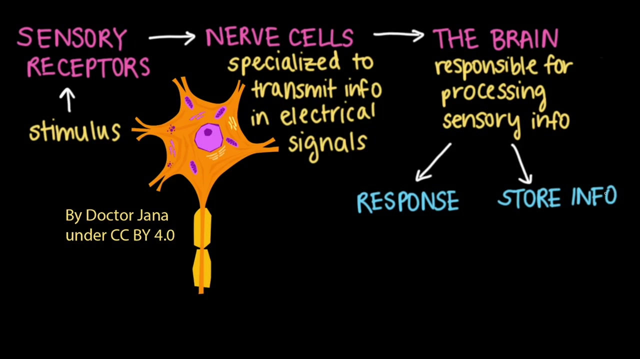 nerve cells. So then, what happens after a sensory receptor receives the information? it passes this information along a nerve cell, troops are immediately 주고 progress, 모든 cells from different nerves to the brain, so that this information is moves in this direction in order and due to the entrenment system, As we connect to the brain, we withstand the 생각이. 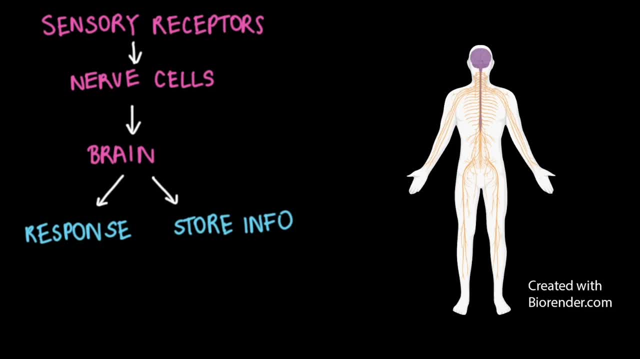 heartbeat. Our attention goes on and onto the brain with our brain and our ear expandings. Here's a picture of a nerve cell which is specialized to transmit information in the form of electric signals. These signals are transmitted along nerves to the brain, which is then responsible for.